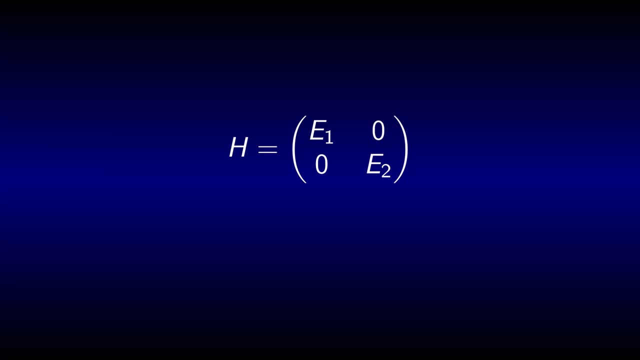 purposefully restricted it to only two states, and those are already diagonalized. Now imagine a second hydrogen atom keeping our first one company. Individually, it is described by exactly the same Hamiltonian. but once they come close, it is possible for our electron to hop into the unoccupied 2s orbital of the other atom. 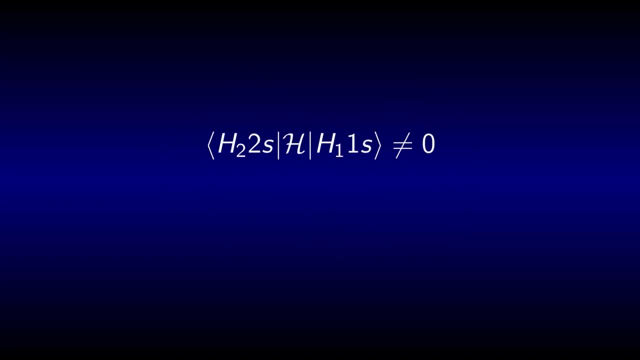 This is possible because the matrix element of the Hamiltonian between the two wave functions does not vanish. Again, with the knowledge of the form of the Hamiltonian and the wave functions, it is in principle possible to calculate the form of the Hamiltonian between the two wave functions. 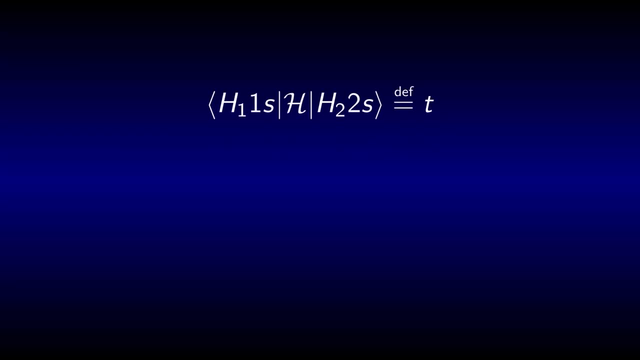 We can calculate the value of this matrix element, but for now let's just assume we had done that and call it T. This is often called the hopping amplitude, Because the Hamiltonian, as the operator corresponding to the energy, is required to be Hermitian. the transposed element has to be the 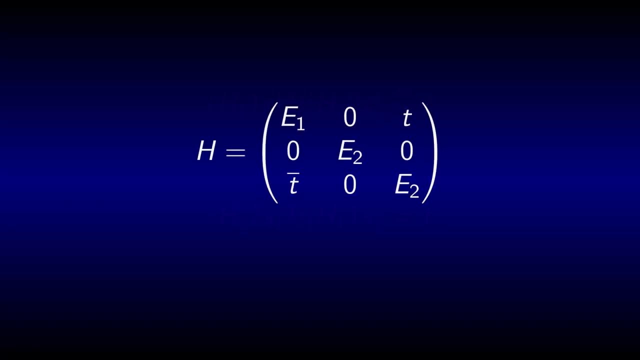 complex conjugate of T. So now the Hamiltonian for one of the electrons looks like this: It is in principle also possible for the electron to get from the 2s orbital of the second atom to the 2s orbital of the first atom. but we'll ignore this interaction for now, Just as we ignored that. 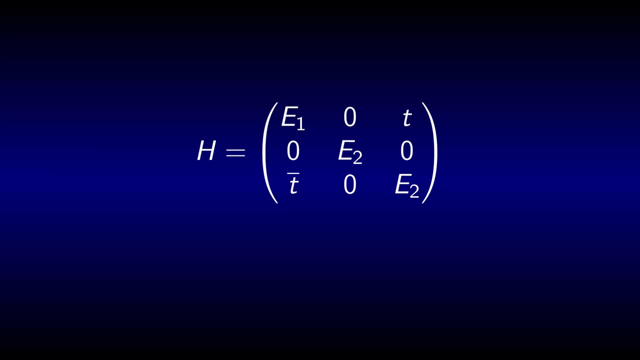 the energies might change under the influence of the second proton entering the scene, Because the electron has, in this approximation, still no chance to get to the 2s shell of the first atom. we will ignore this orbital in what follows. Our two basis states are then: 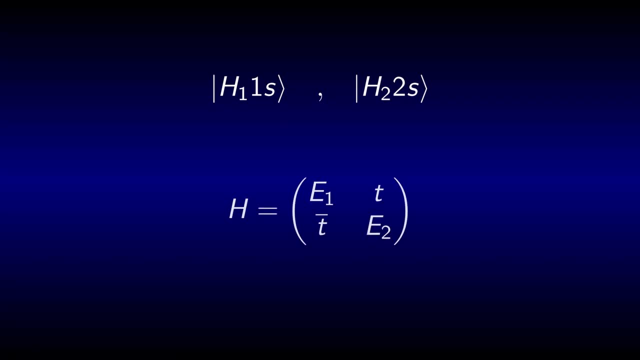 H1 1s and H2 2s and the Hamiltonian has a nice and simple form. Over time, due to interactions, the system will try to get to its ground state, the eigenstate with lowest energy. We are interested in the energy of that ground state, so let's do some algebra. 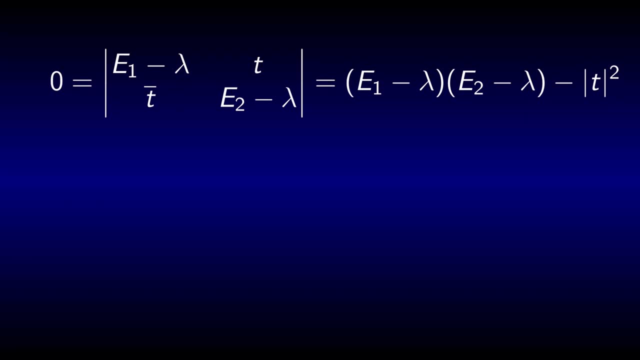 The eigenvalues are given by the zeros of the characteristic polynomial which is the determinant of our matrix, minus lambda times the unit matrix For a 2 by 2 matrix. this is easily calculated. Let's analyze this a bit. The coupling gives us two energies which still have the same midpoint. 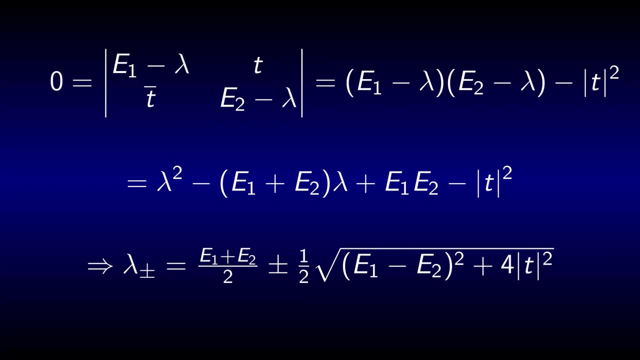 e1 plus e2 over 2.. If t was zero, we would just get out e1 and e2, as expected. but if t is non-zero, then the peaks split farther apart. If the two energies are very far apart, then t has next to.